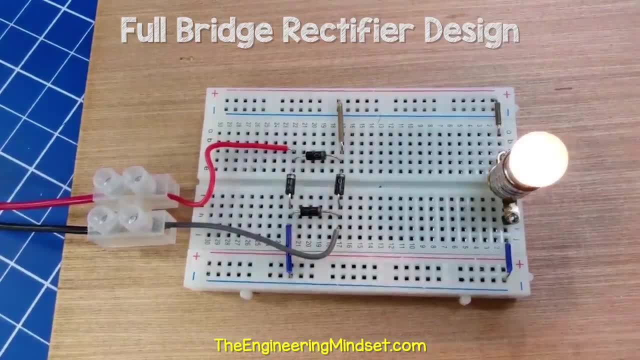 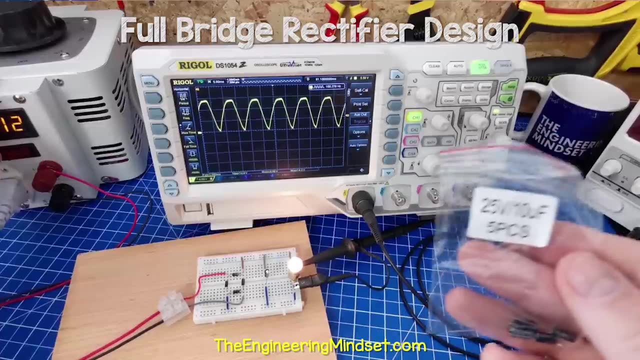 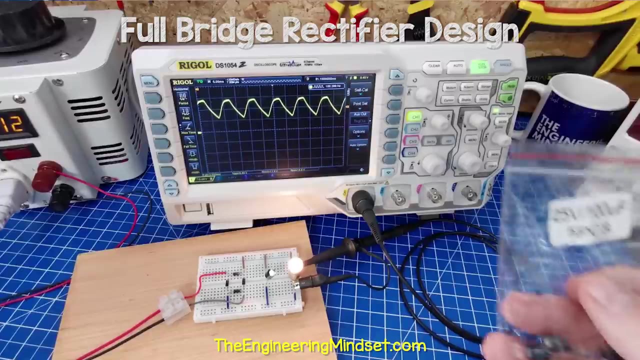 and powering the LED during the interruption interruptions In this circuit I have a lamp connected as the load. The oscilloscope shows the rippled waveform. When I add a small 10uF capacitor, we see that it makes very little difference to the waveform. When I use a 100uF capacitor, we see the dip is no longer down to. 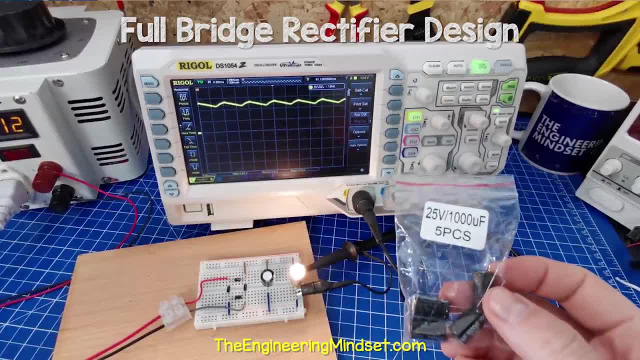 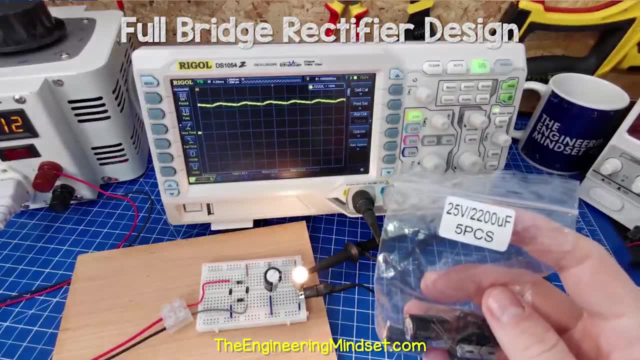 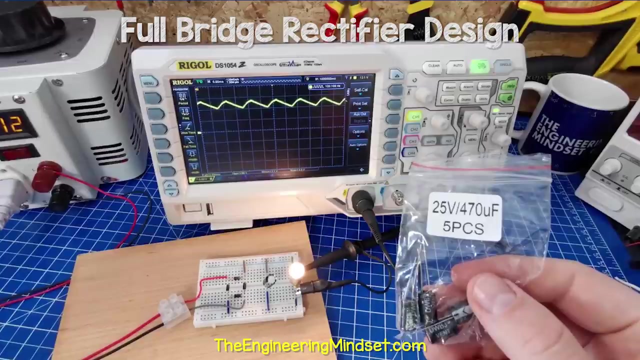 0V At 1000uF the ripple is very small. At 2200uF it's nearly completely smooth. This would be fine to use for many electronic circuits. We could use multiple capacitors also. Here we have a 470uF capacitor, which has made some difference. but if I use two capacitors, 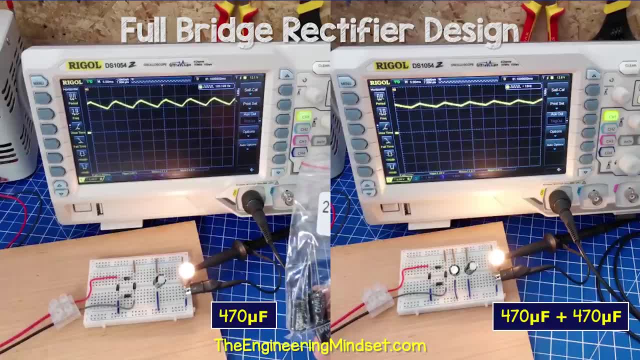 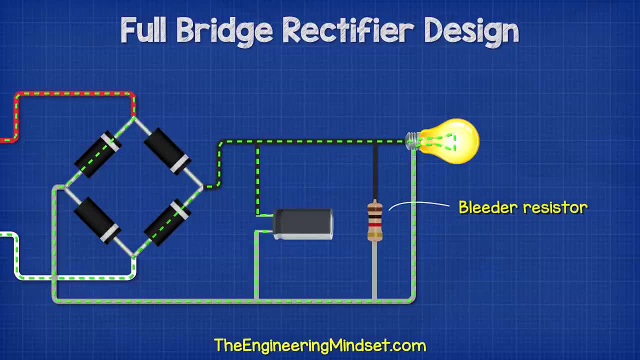 in parallel, we see the waveform is much more improved. When using a capacitor, we need to place a bleeder resistor across the output. This is a high value resistor which will drain the capacitor when the circuit is off. to keep us safe, Notice. 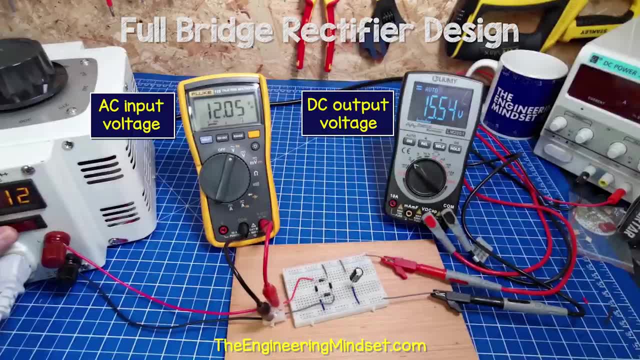 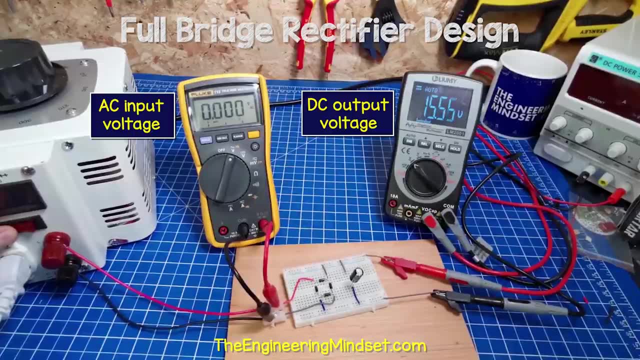 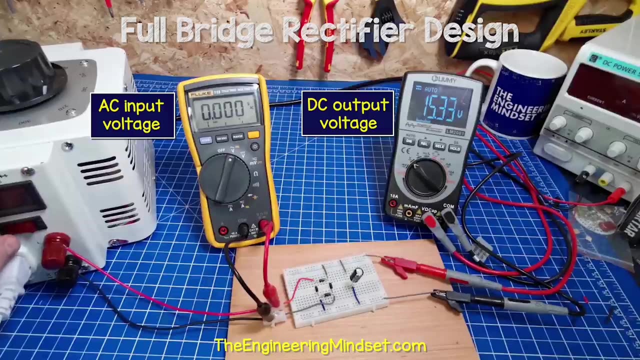 with this circuit that when I switch it on the capacitor charges quickly to over 15V, But when I switch it off the DC output is still at 15V because there is no load, so the energy is still stored in the capacitor. This could be very dangerous if the voltage is high In this example. 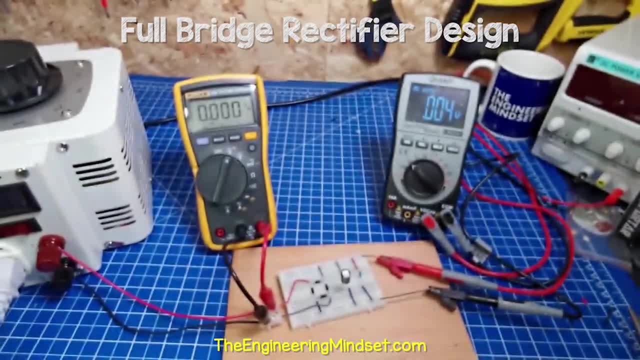 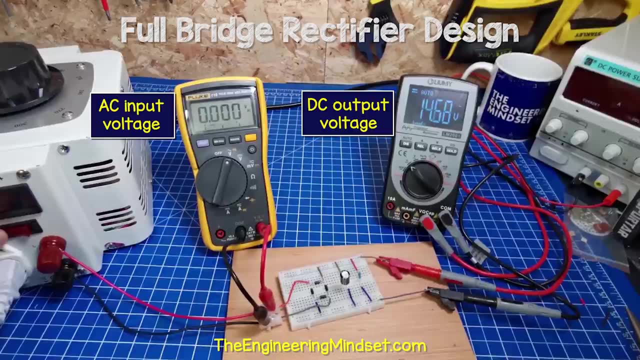 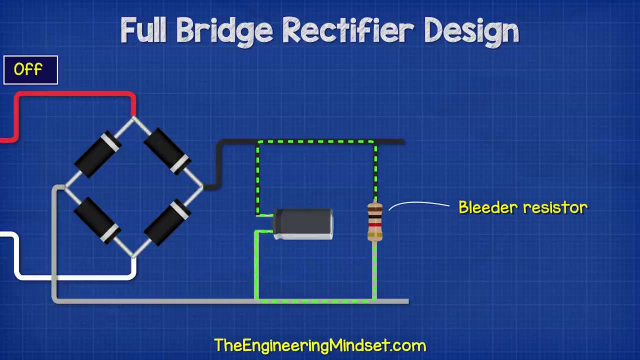 I place a 4.7kΩ resistor across the output, We see the capacitor charges up to 15V and when I switch it off, the capacitor quickly discharges. The electrons are flowing through the resistor, which discharges the capacitor. We can also see that without a capacitor, the output voltage is lower. 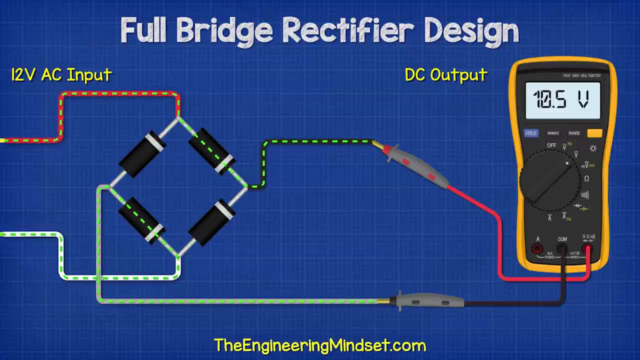 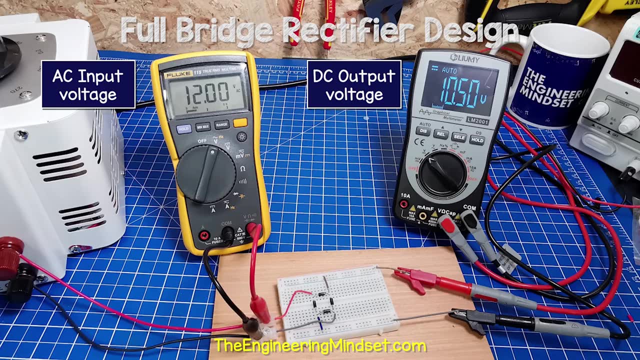 than the input voltage because of the voltage drop of the diodes. Here we have a simple 4-wave bridge rectifier. On the input we see there is 12V AC. On the output we have 10.5V of DC. The voltage on the output is lower because of the diodes Each diode has. 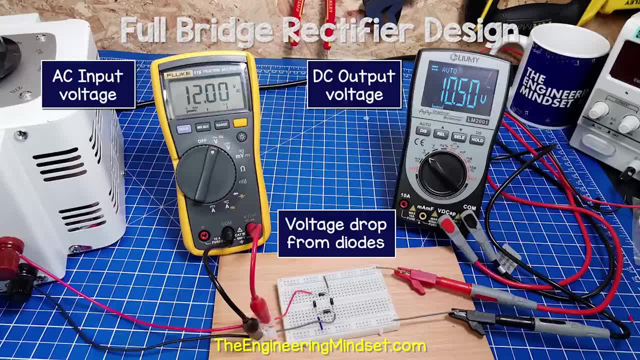 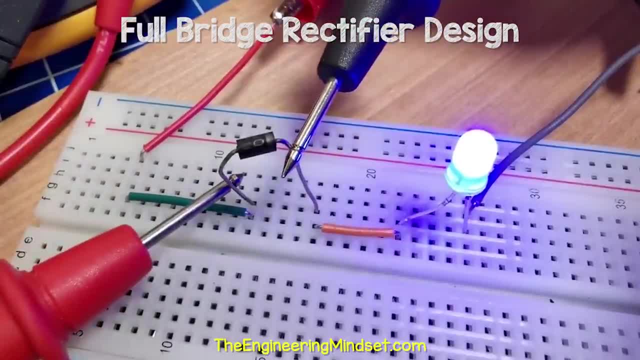 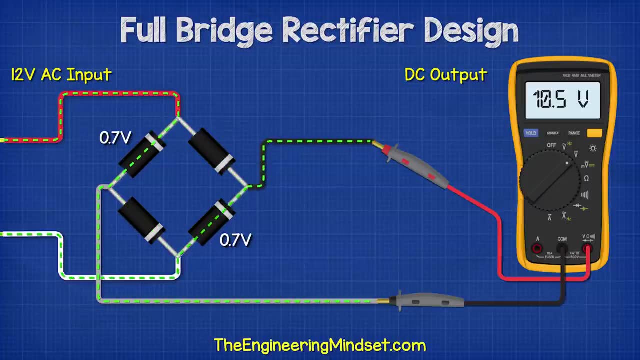 a voltage drop of around 0.7V. If we look at this circuit with a diode and an LED, we can measure across the diode to see a voltage drop of around 0.7V. The current in our full bridge rectifier must pass through two diodes on the positive half and two diodes on the negative. 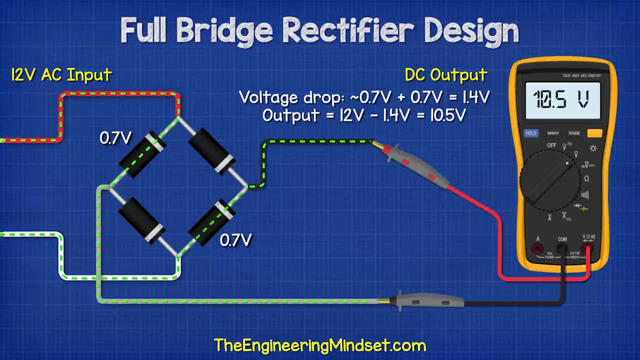 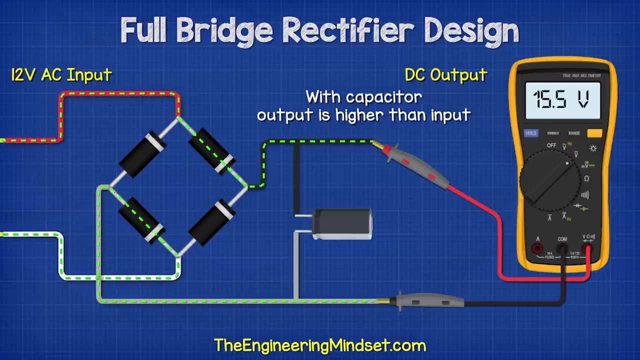 half. So the voltage drop combines and is around 1.4 to 1.5V. So that is why the output will be reduced. However, if we were to connect a capacitor across the output, we will see that the output voltage is now higher than the input voltage. How is that possible? That's. 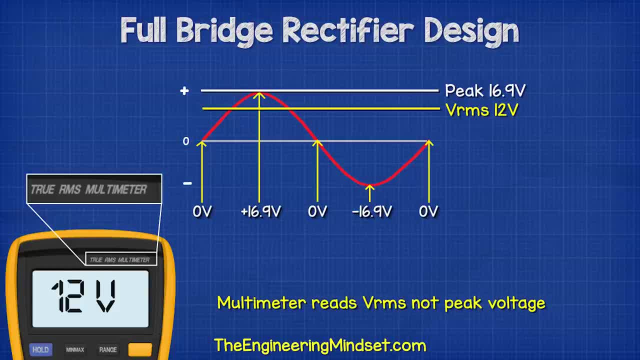 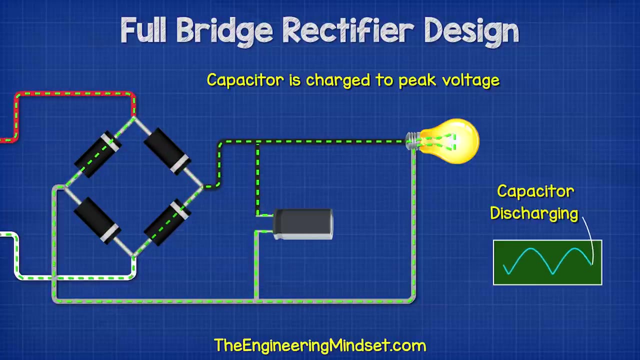 because the AC input is measuring the RMS voltage or the root mean squared. This is not the peak voltage. The peak voltage is 1.41 times higher than the RMS voltage. The capacitors are charged up to the peak voltage and then release. There will be a small voltage. 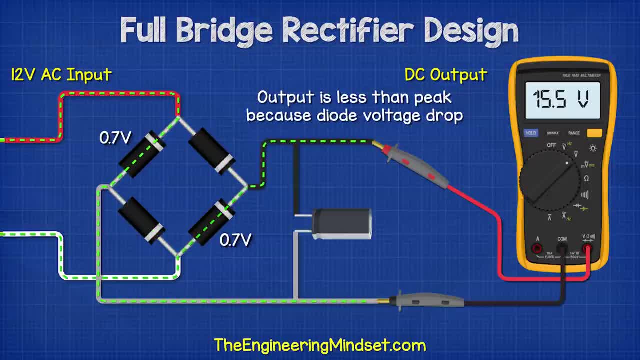 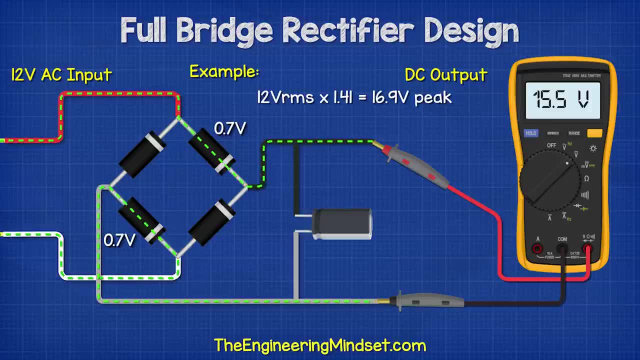 drop because of the diodes. So the output is less than the peak input, but it will still be higher than the RMS input. For example, if we had 12V RMS on the input, the peak voltage would be 12V multiplied by. 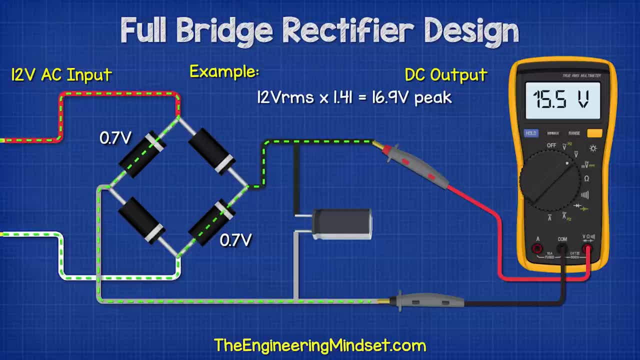 1.41, which is 16.9V. There will be a 0.7V drop here and here, so 16.9V subtract 1.4 is 15.5V. The capacitors are charged up to this voltage. This is only the approximate answer, though. 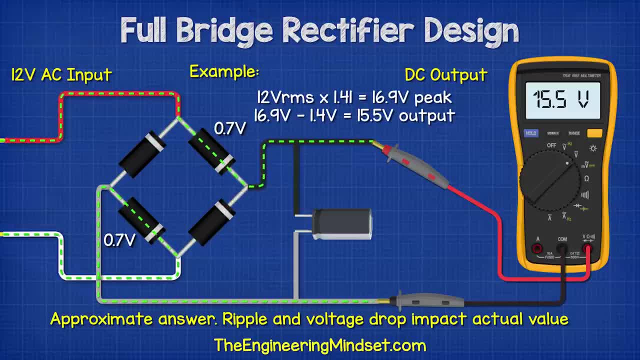 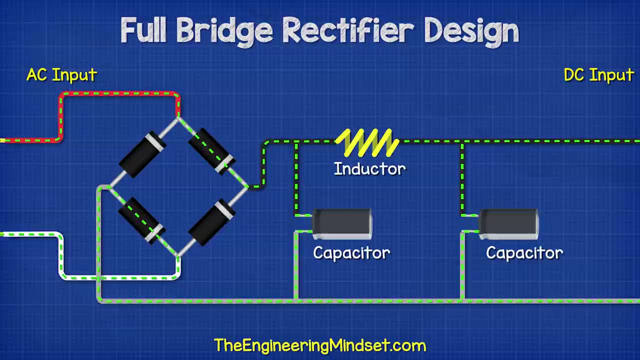 The amount of ripple and the actual voltage drop of the diodes will cause it to be slightly different in reality, but we can see that the output is higher than the input. Another common filter is placing two capacitors in parallel with a series inductor between. 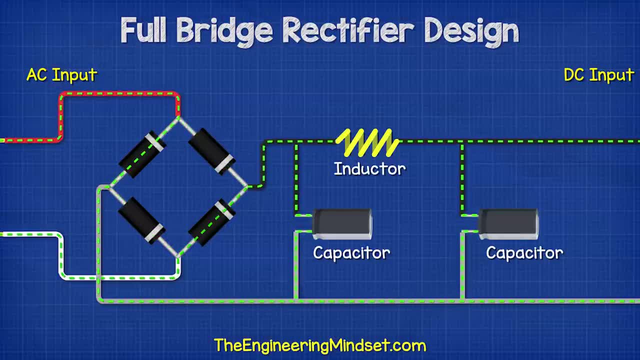 these. This is used for circuits with larger loads. The first capacitor smooths the ripple. The second capacitor smooths the ripple. The third capacitor smooths the ripple. The third capacitor smooths the ripple. The third capacitor smooths the ripple. The fourth capacitor smooths.